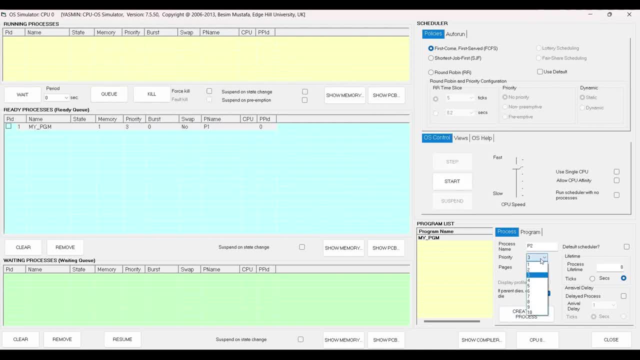 process P1 is being created Now. let us create process P2 with priority, as let us assume as 4, and let us create it. And let us create process P3 with priority, as maybe let us take it as 1.. And finally, process P4: let us create priority as 2.. 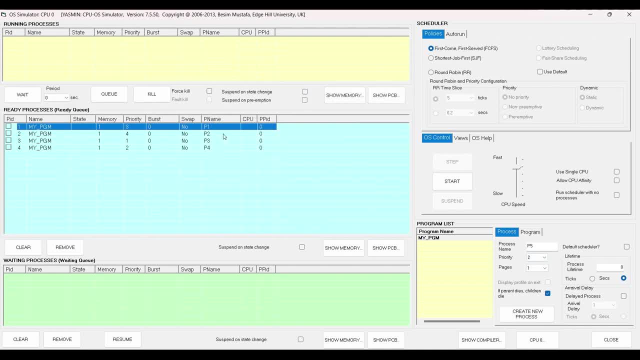 So now I have created all the 4 process and, as the order I have created them, they have been loaded in the ready queue in the same order. So now let us start the simulation. You see, the process 1 is being served here in the ready queue. 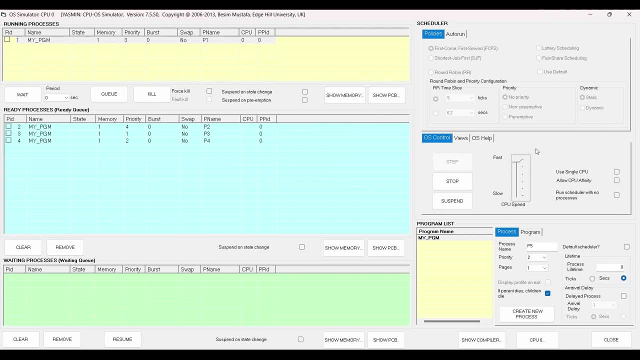 Let us increase the CPU Speed. So, as you notice in the simulation and the process was served in the order it was created and no other overrides happened, even though the priorities were different and, like, process 4 had a better priority than process 1 or any other project. 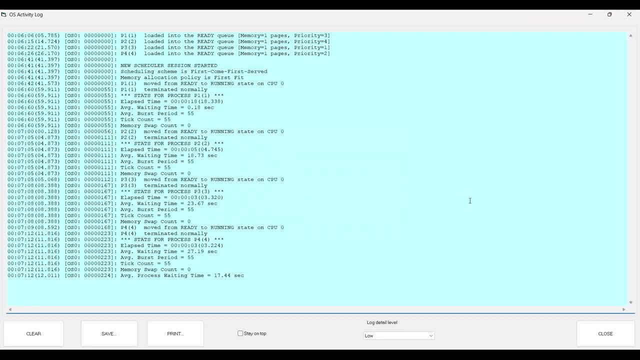 other things. For more details, let us go to the log. We see the log here and we see that the process 1 was loaded into the ready queue, process 2,, process 3,, process 4 and we see the priorities as well here Now, when the scheduler was started. 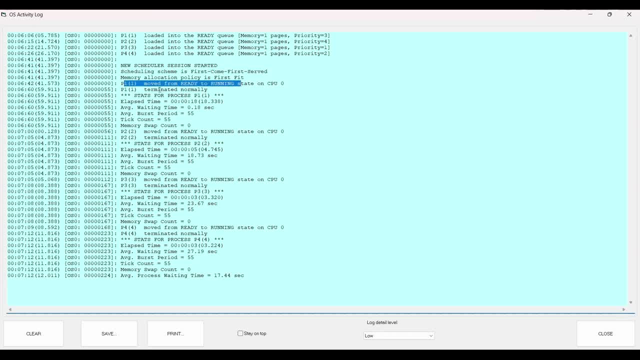 we scheduled. of course we used the first come, first serve. Now we see the process. 1 was the one which first moved from ready queue to running state and then it was terminated. It took some time of 18 seconds, so it waited for 0.18 seconds before it could start. After that, we see process. 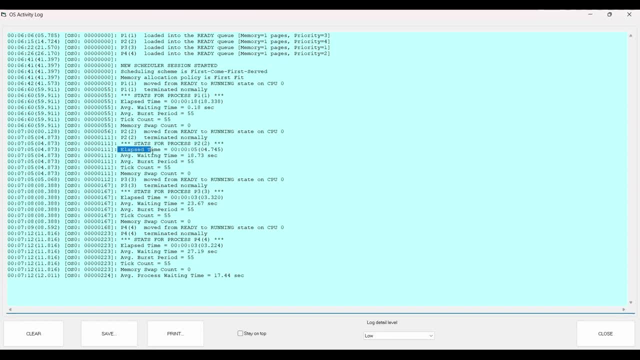 Q2 started and its total time for it to be evaluated was somewhere around 0.5 seconds, but of course it had to wait for 18 seconds before it got its time to go ahead to the CPU. Same thing happened with P3 and P4 here respectively, So we see in this simulation that there was no 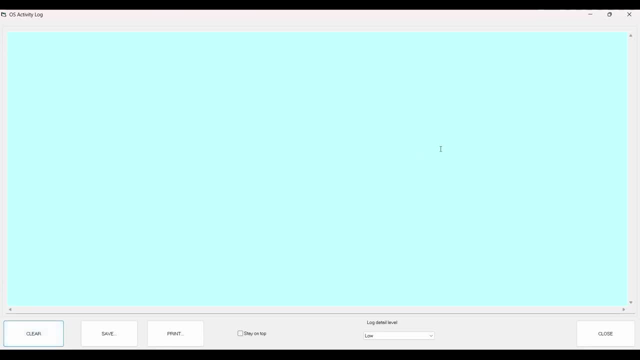 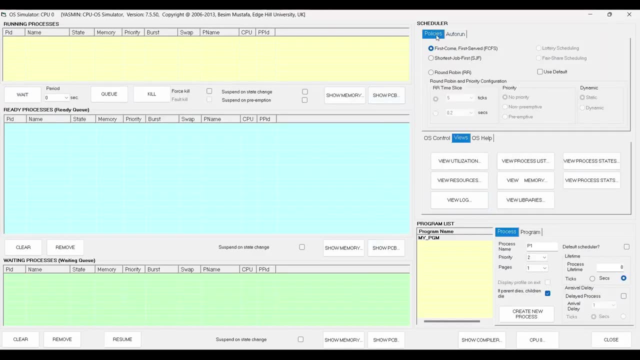 impact of priority or any other thing. even though we added some priority in the first come, first serve algorithm, Now let us just go and let us reset the program and let us go back to the OS options. Now let us start the second simulation. I will create a process P1 with priority 3 and for now, 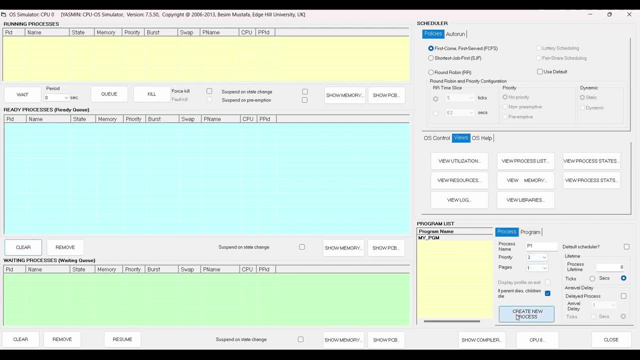 it is 0 and the arrival time is 0, so there is no arrival time. So I will just create the process. I will take process P2 and maybe I'll take the priority as 4 and let us take that it was delayed by 4 seconds. Let us create the process. So now we see there are two different boxes here. 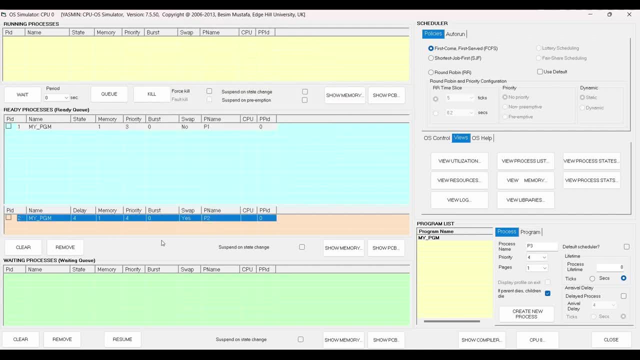 there is one which is the ready queue and then there is another queue which is here, which is Marvin Red. So the process to get ready queue is 0, but in this scenario it is 0.25 seconds. So, process which has no delay and which are at the ready queue are being loaded here and 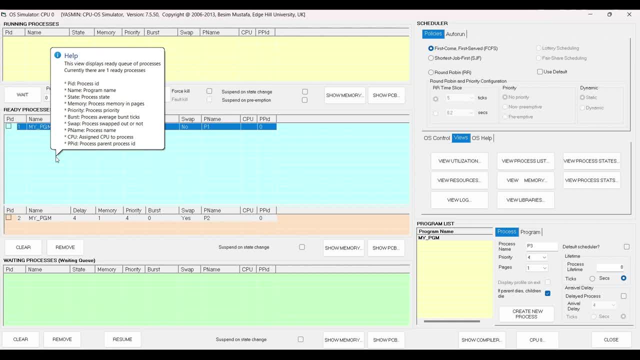 the process, which have some delays in arrival. basically, it means that it will be created after certain time in the future, but for the purpose of simulation they have been created beforehand and are kept in this queue here marked in red, so that we can see it and we 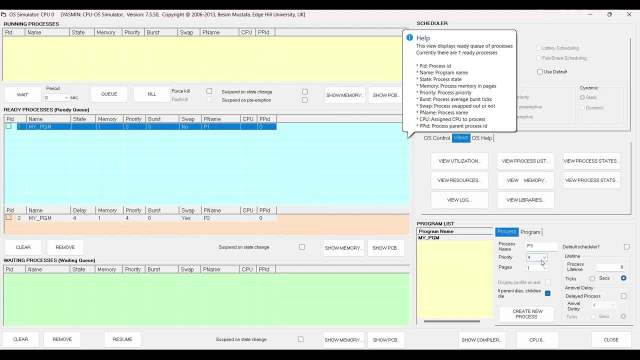 can know how exactly it works. Now let us create a process P3 with priority as 2, and let us take the arrival time as 2 and let us create it. and then let us finally take process P4 with priority 1, and let us 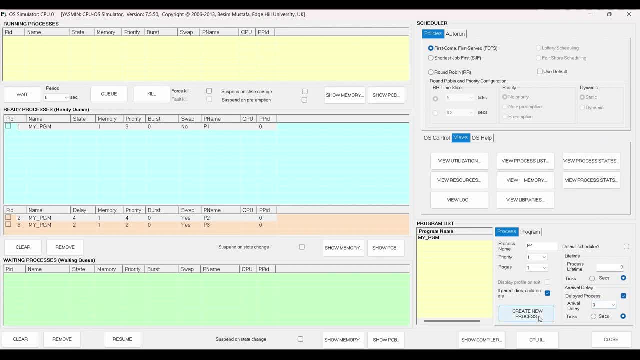 say, it got delayed by 3 seconds. so now see here it is. so I have process P1, which has no delay, then we have process P2, which has 4 seconds of delay, process P3, which has 2 seconds, and process P4, which has 3 seconds of delay. 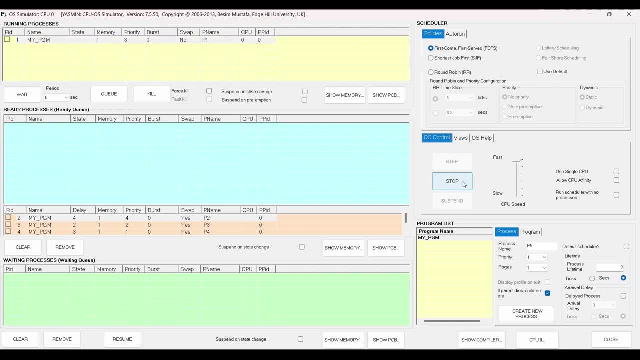 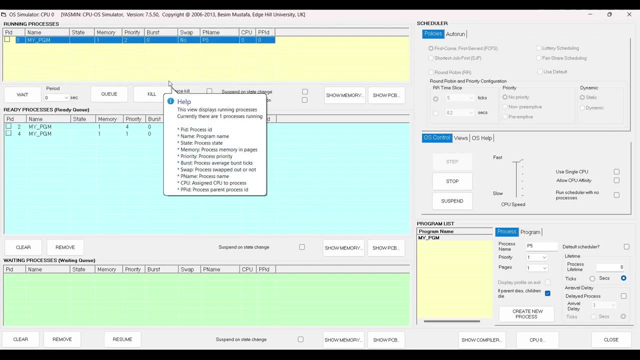 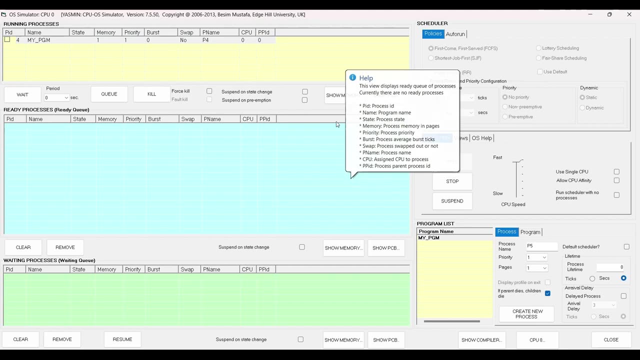 So now let us start the simulation. So now, let us start the simulation. So now let us start the simulation. We see, process P1 went inside and then process the other process came along inside the ready queue and are being served. So finally, everything is over.